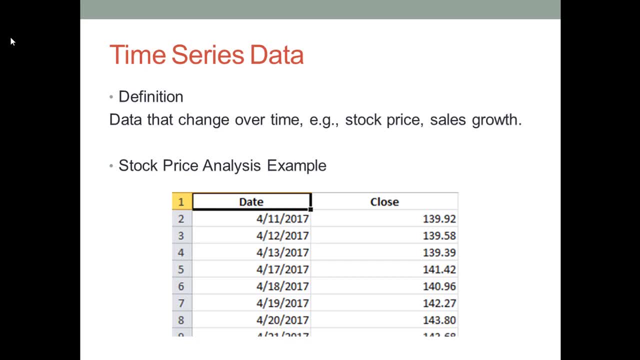 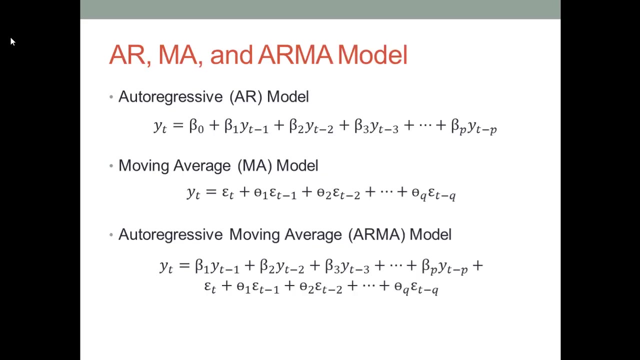 the relationships among data values over time. This is the purpose of this lecture video series. We want to learn how to use analytical model to analyze data over time. From a mathematical standpoint, we can present time series data in three ways. The first one is called an autoregressive model, The 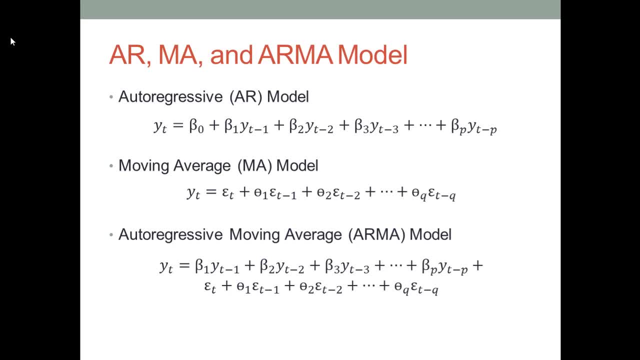 second one is called a moving average model. The third one is a combination of autoregressive and moving average models. Let's talk about them one by one. The autoregressive model believes that Rome was not built in one day. The data value at the current time spot is: 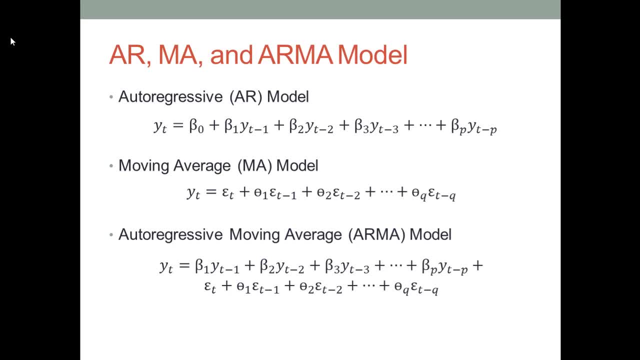 built on top of the data values at the previous time spots. For example, today's stock price is built on top of the stock prices in previous days. If we use the autoregressive model to analyze a time series data, our job is to identify. 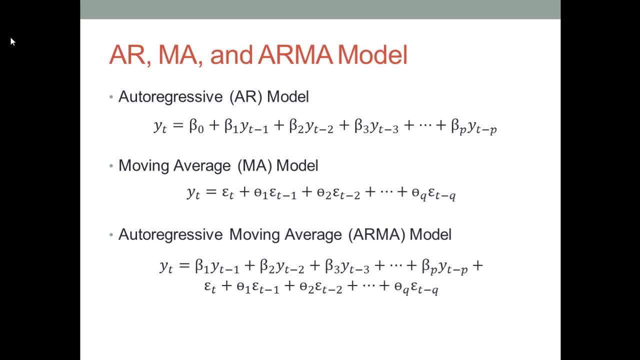 how many days we need to look back in order to forecast the current value? What should be the value of the current value? What should be the value of the current value? What should the price of product be? How should the price of product be? Height, Quantity or time? 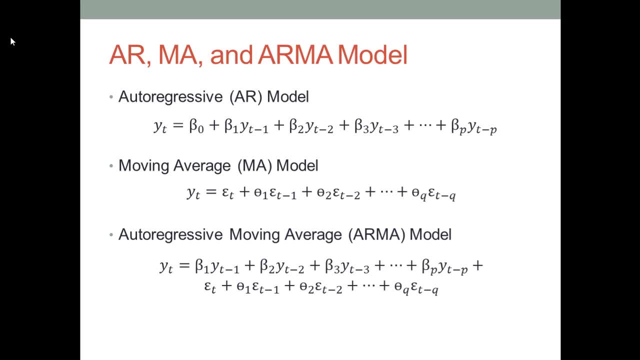 appropriate How to flying Whatattle value for coefficients like beta 0,, beta 1,, beta 2 and so on. This is an autoregressive model. In practice we usually use a short name, ar, to represent autoregressive model. The second model is called the moving average model. 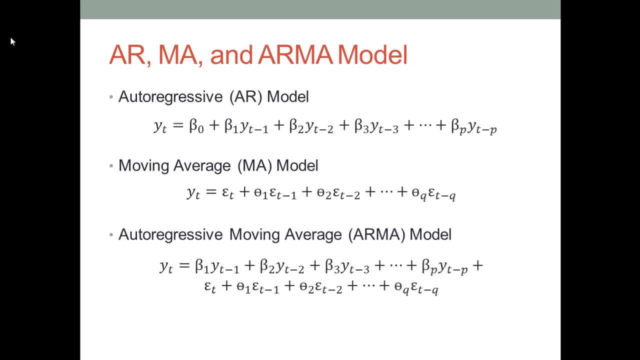 This model believed that the current data value is a result from previous unexpected events. For example, the current stock price can be a result of unexpected events like the US election results, the COVID-19 pandemic, a better sales revenue, the CEO change of the company and so on. 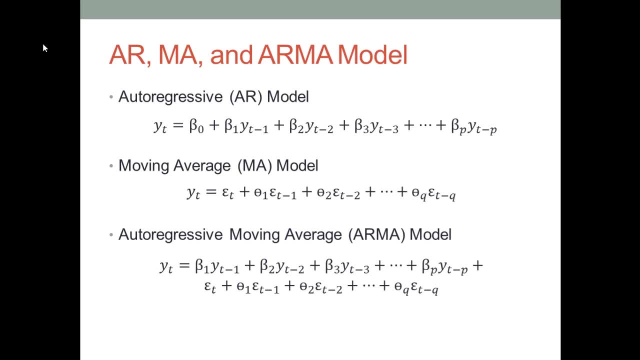 If we use the moving average model to analyze time series data, our job is to identify how many days of unexpected events we want to look back to forecast the current value. What should be the values for the coefficients like theta1, theta2, and so on? 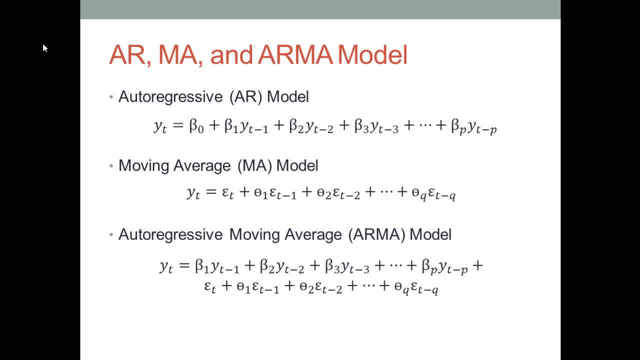 In practice, we usually use a short name MA to represent moving average. The third one is a combination of AR and MA model. This model believes that both AR model and MA model have valid points, So why don't we combine both models together in order to forecast the current value? 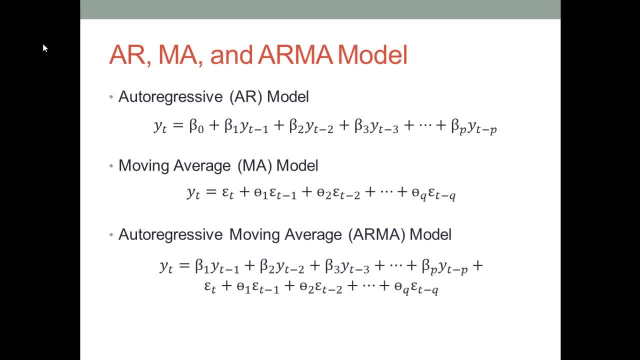 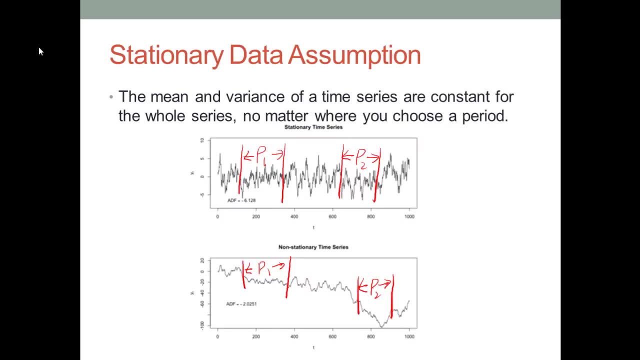 In practice, we use a short name ARMA to represent the autoregressive moving average model. No matter which model you plan to choose, the first step is to make sure the time series data follows a stationary data assumption. This assumption believes that a time series data set should have a constant mean and a constant variance. 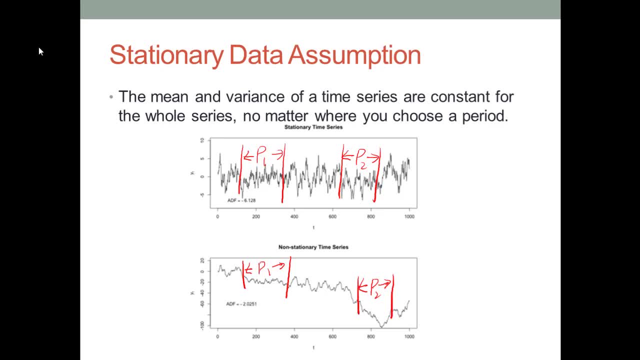 The constant mean and variance should be the same throughout the entire time series, No matter where you choose. this assumption will be given in the set times. In practice, when we are given a time series data set, the very first step is to draw the time series on a plot chart. 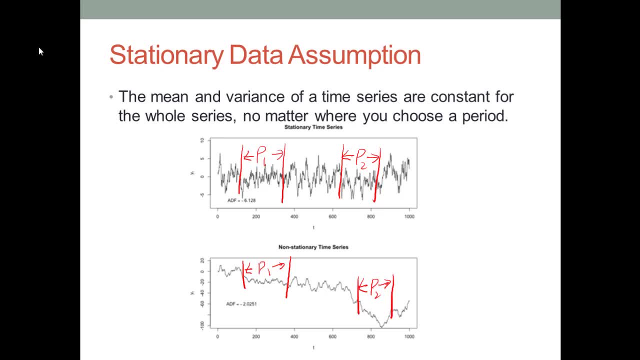 If a time series follows the stationary data assumptions, the time series should be pretty flat. The data value should change around a central value, as you can see in the top chart of this slide. If the time series is not a stationary dataset, then you should have an obvious trend either decreasing or increasing in the plot chart, like you can see in the bottom chart on this slide. 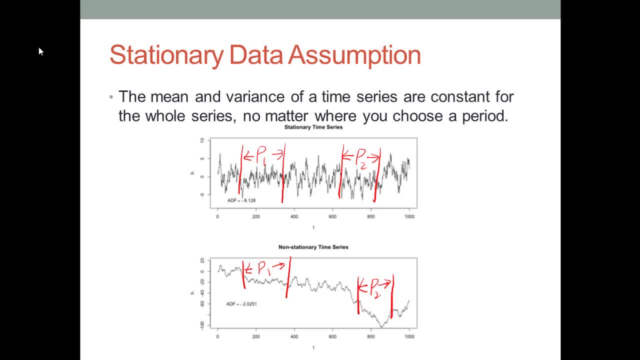 The bottom chart is not a stationary dataset. Why, If I randomly choose two periods, let's say p1 and p2, obviously you can see the mean of p2 is less than the mean of p1 in the bottom chart. So the time series in the bottom chart is not a stationary dataset. 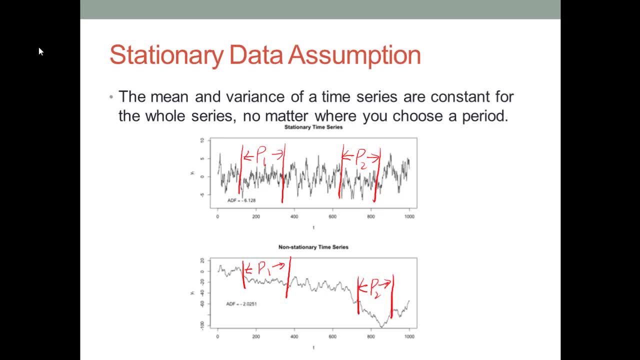 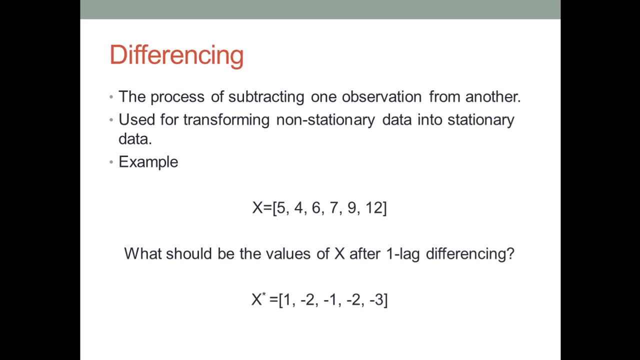 When we face non-stationary datasets. what can we do to transform this non-stationary dataset into a stationary dataset? In practice, we use a technique called differencing to do the data transformation. Simply speaking, differencing means that we want to subtract previous values from the current value. 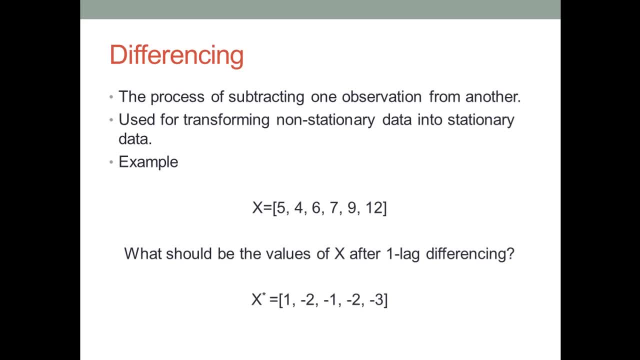 On this slide we are given a dataset x. Someone asked us to do one-leg differencing. What this means is we want to subtract 4 from 5.. So we subtract 4 from 5.. Then we subtract 6 from 4.. 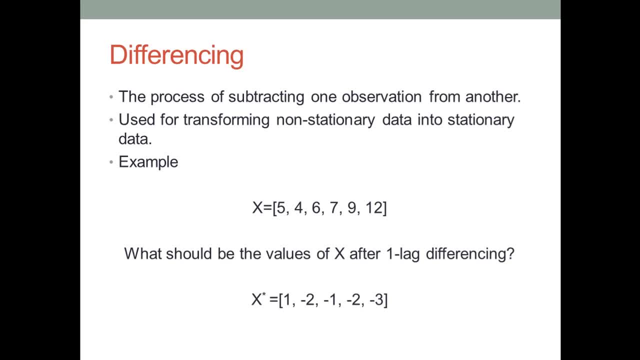 Then we subtract 7 from 6.. Then we subtract 9 from 7.. Then we subtract 12 from 9.. Eventually we come to the last data value, 12.. We don't have previous value to subtract from 12.. 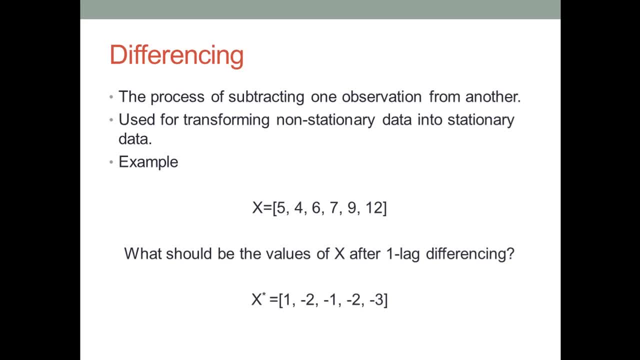 So we will just stop at the final value 12 and exclude 12 from the final value 12.. Finally, we get the result from the one-leg differencing x-star, as you can see at the bottom of this slide. Some classmates may say this is simple. 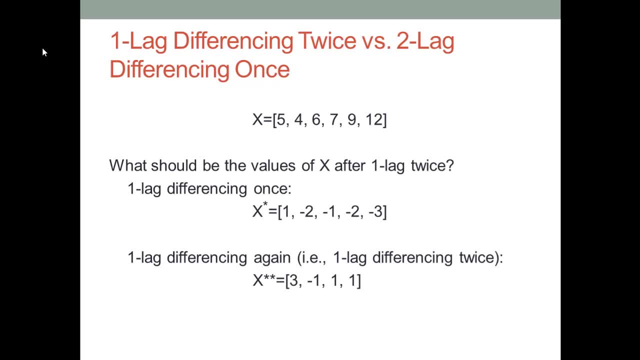 But in practice someone may challenge you to do one-leg differencing twice or two-leg differencing once. Let's talk about them one by one. We just did one-leg differencing in the original dataset x. We get the one-leg differencing once. result: x-star. 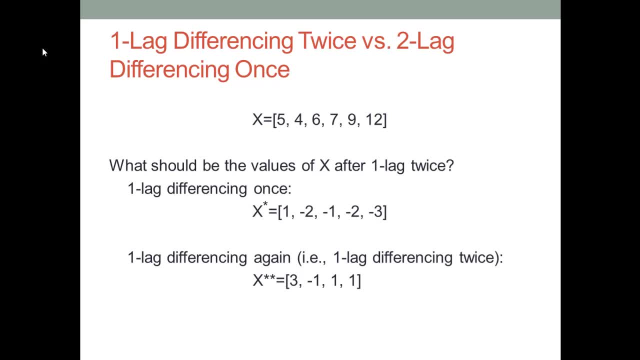 One-leg differencing twice means in the x-star dataset we need to subtract the values again. What we need to do is to subtract negative 2 from 1.. Subtract negative 1 from negative 2.. Then we want to subtract negative 2 from negative 1.. 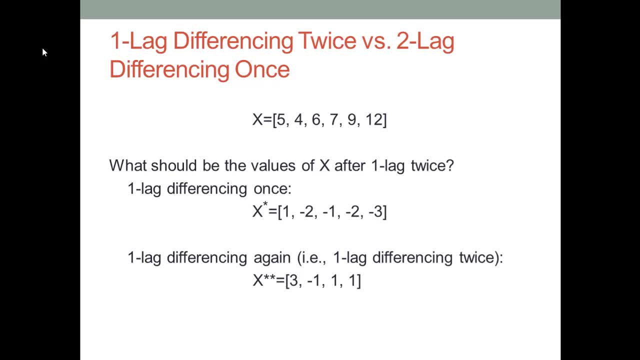 Then we want to subtract negative 3 from negative 2.. When we come to the final value- negative 3 in x-star, we don't have previous value to subtract, So we will stop at negative 3.. Eventually we get a new result: x-double-stars. 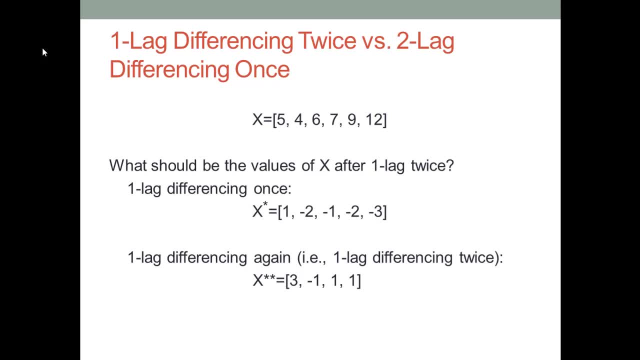 x-double-stars is the result of doing one-leg differencing twice. Two-leg differencing means we need to subtract the data value two days back from the current value In the original dataset. if we want to do two-leg differencing once, we need to subtract 6 from 5.. 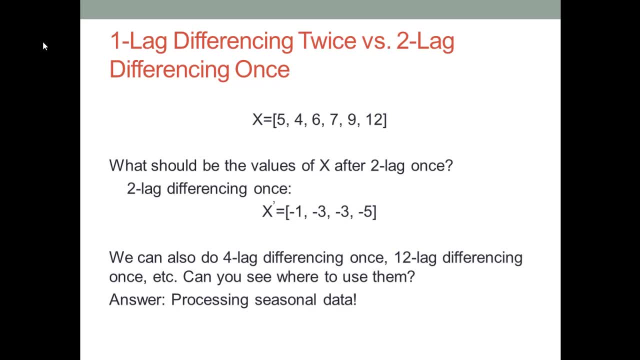 Then we subtract 7 from 4.. Then we subtract 9 from 6.. Then we subtract 12 from 7.. When we come to the value 9, we don't have a value two days back, So we'll exclude 9 and 12 from the final results. 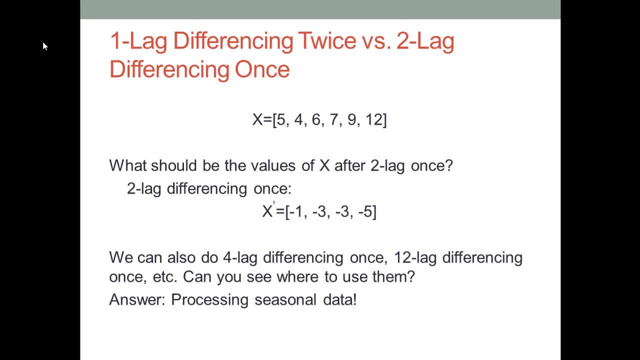 Eventually we get the results from a two-leg differencing once x-prime. as you can see on this slide, If we can do two-leg differencing, we can also do four-leg differencing, twelve-leg differencing. Can you see where we use four-leg differencing and twelve-leg differencing? 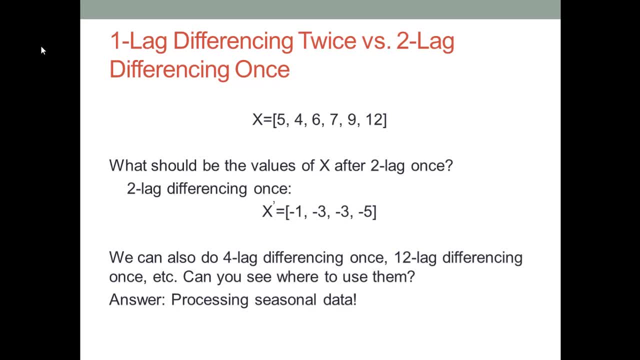 Yes, we can use them to process seasonal data. We need to transform seasonality into a stationary dataset as well. In the next few lectures, I will talk about all of these things. I will talk about all of these techniques in more detail. 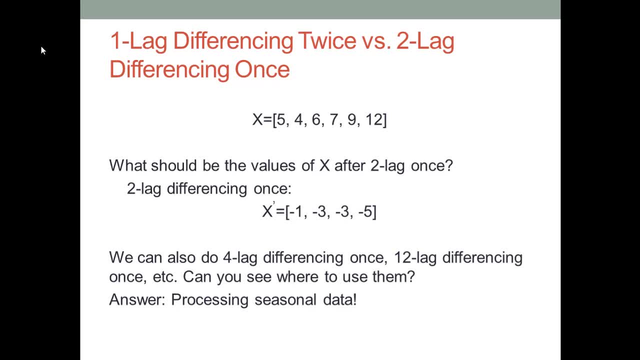 Fortunately, we don't have to do differencing by hand. As long as you figure out what types of differencing you want to do, how many times you want to do the differencing, you can teach the software and let the software do all the labor work.